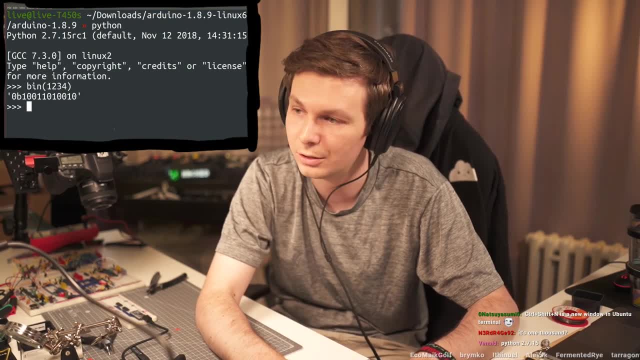 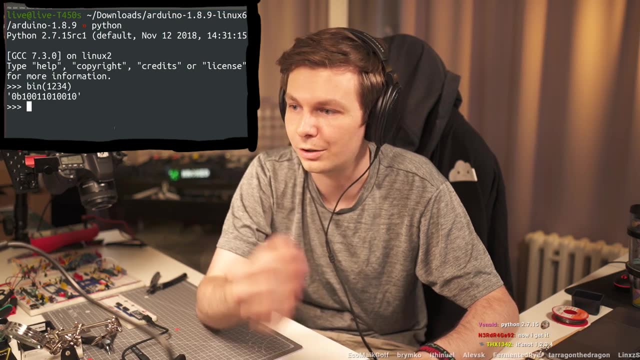 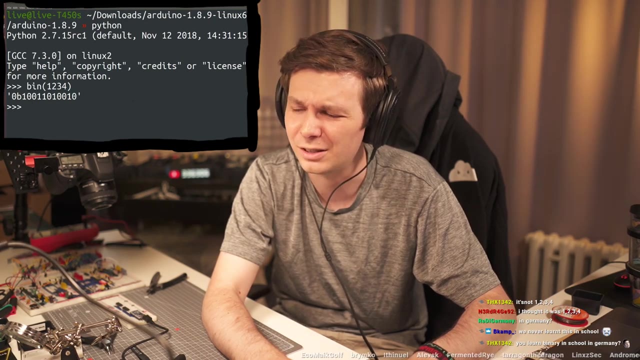 in decimal converted to binary, is one zero zero, one, one zero, one zero zero. didn't you have binary numbers in school? we learned that like in sixth grade or so. oh, you thought it was one, two, three, four. well, yeah, obviously not in germany. yeah, i had that in in like sixth grade, maybe seventh. 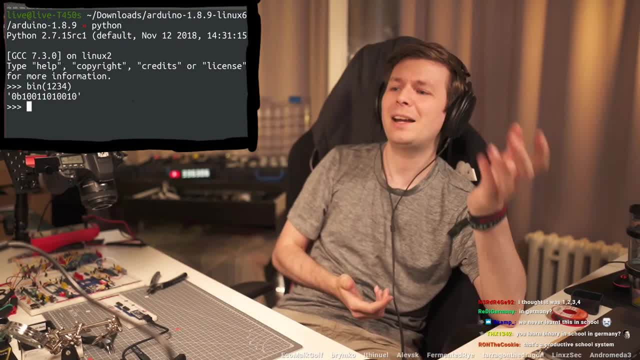 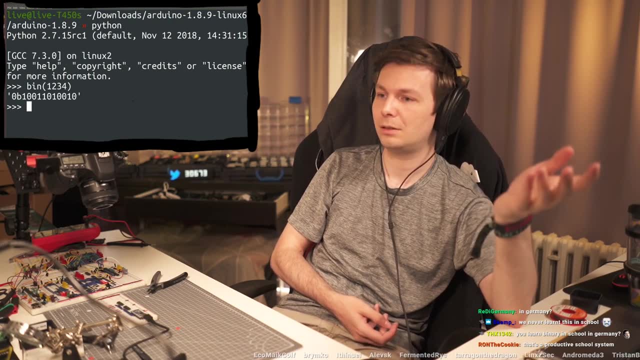 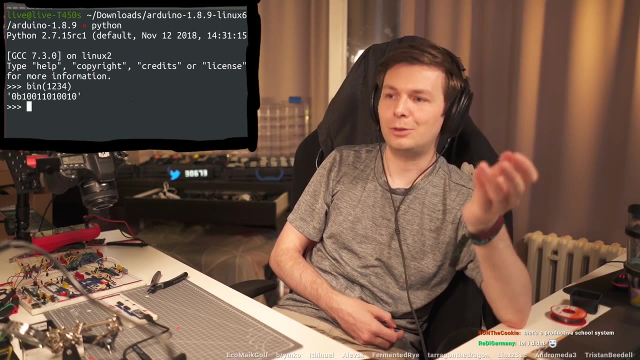 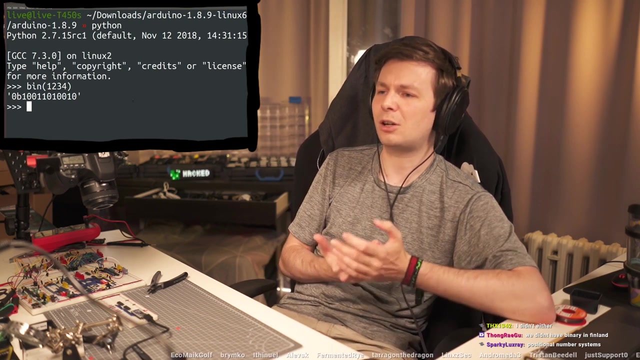 grade or so yeah, it takes, but we had like a whole. we didn't learn binary. we learned converting into different uh number- what is it called number basis in different bases. we, we did that into hexadecimal. we did that into uh octo. we didn't we did that into like into anything. we learned how to do that like we. so so the the concept, 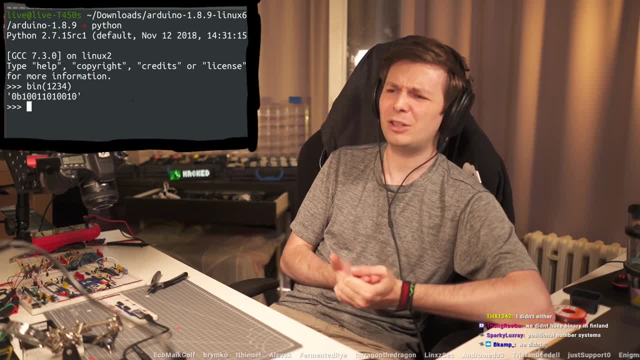 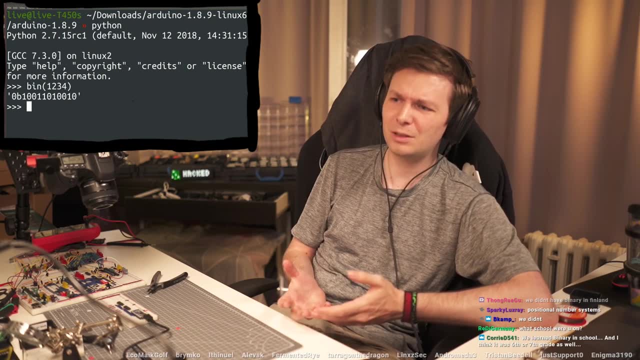 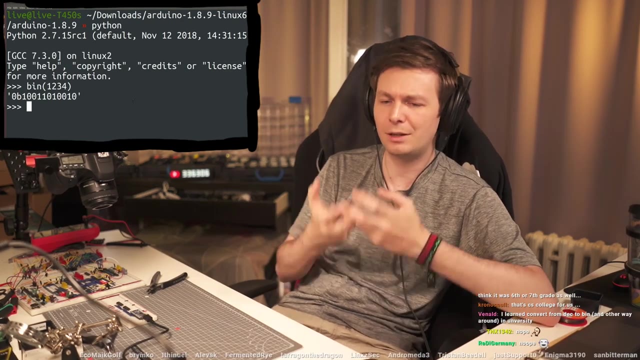 of so in your math class. you never talked about it. there you have a different number base. like you never talked about that we use the decimal system and that you can also represent numbers in different ways. i'm not specifically talking about decimal to binary. that's obviously a kind. 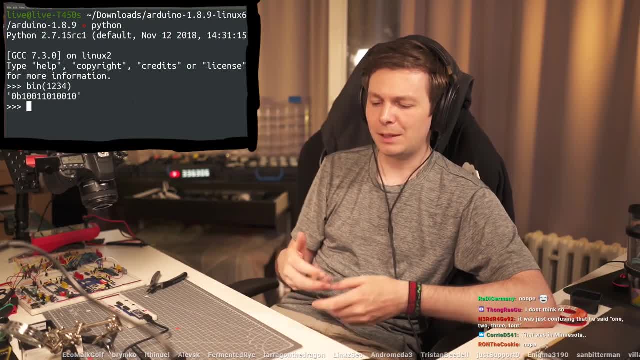 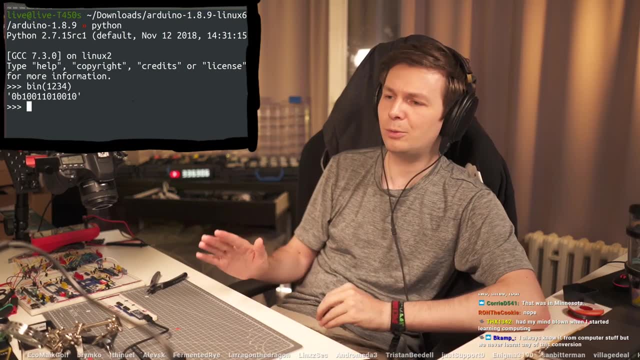 of a thing for for programming, right, but but this concept of having different number base, that there's decimal and other stuff, you don't learn that in school? it's had nothing to do with computer stuff. i'm talking here about just the mathematical concept of representing numbers in a different base. 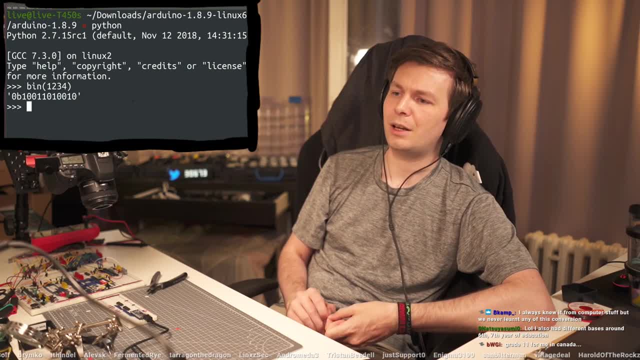 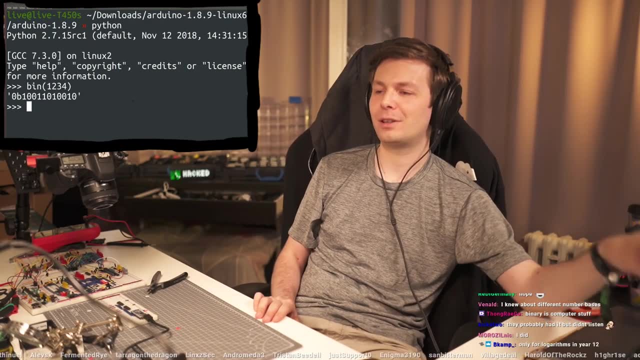 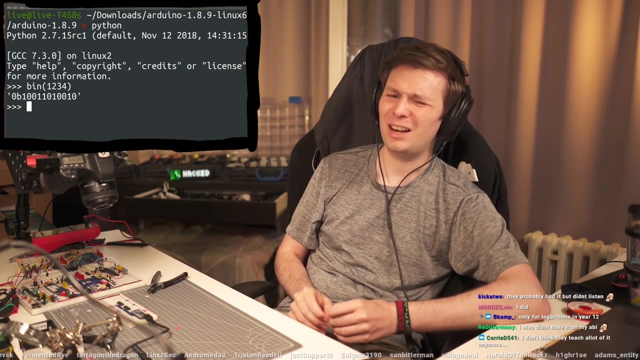 your different bases in sixth or seventh grade. so weighted decimal means what? yeah, maybe somebody didn't hear the difference in maths right, but like probably a lot. like they only understand everything that can be used. if you use a colloquium, yeah, one might understand something else in a certain anchor return. 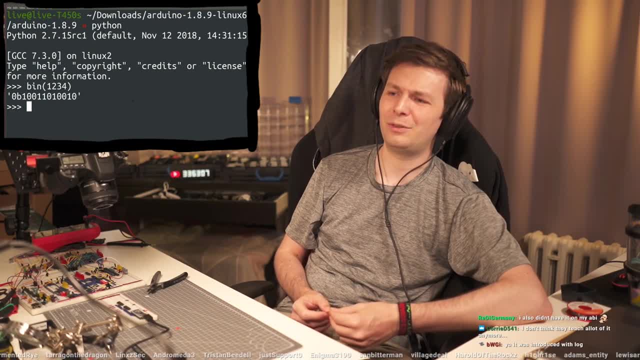 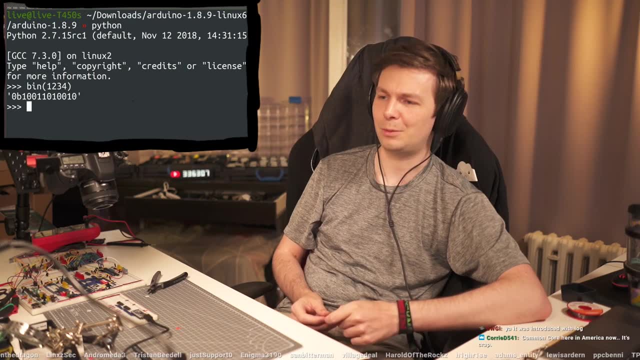 right and yours are something productive, another grade like that, and uh, and there are all kinds of things that can be used in that way, and then the answer is: there information, the things that theώ don't know. that's a later point, as we discussed in eric and victor yesterday about code saying: 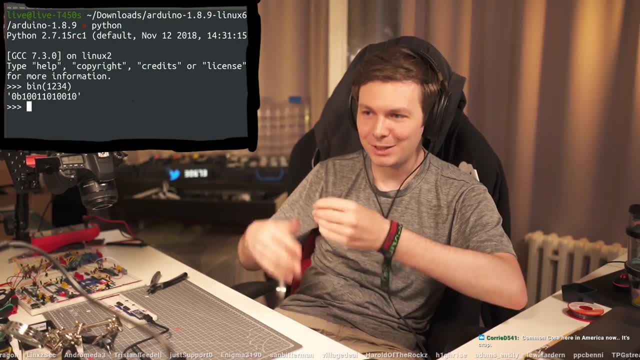 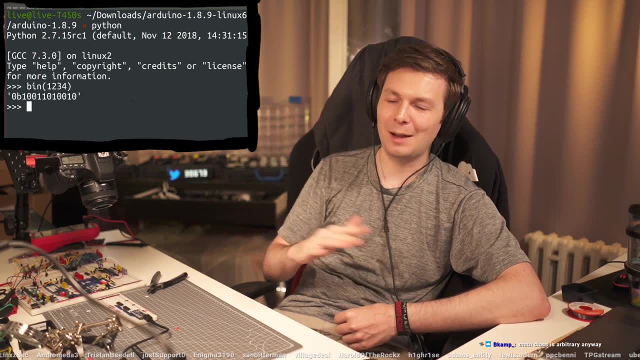 I mean, I don't know the algorithm that you know the steps that you learn in school to convert between those different bases, But I don't remember that at all anymore. right, I, I will, I guess I could, I can, it could get it done.